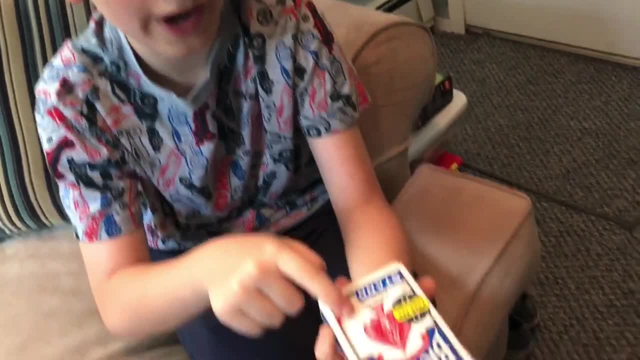 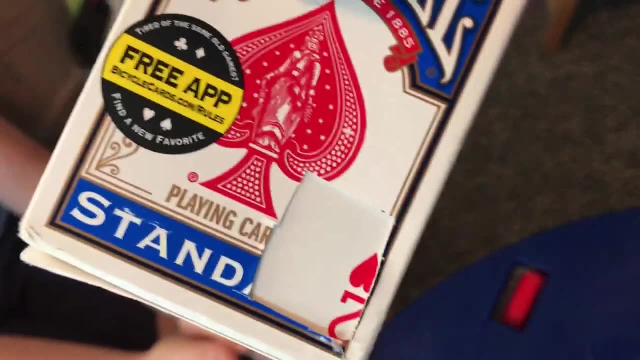 to lift it up to my head. yep, i quickly look right here, since there's a hole in the box. oh, you caught a hole in the box. you can see enough the number and the suit. oh, so you just cut a little square at the bottom of the box. yes, and you look at it quickly. oh, that's why you held the cards up to. 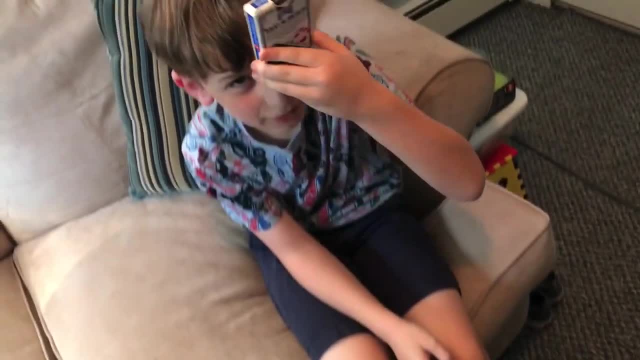 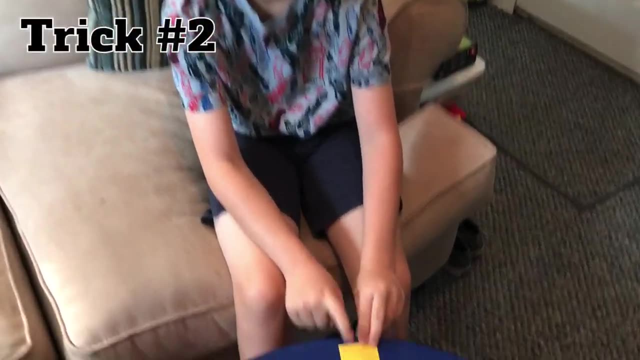 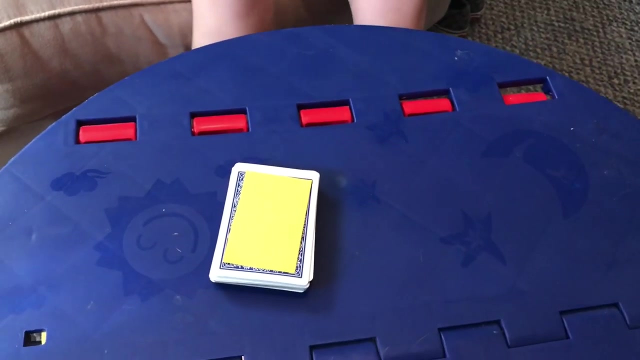 your head when- yes, when- you come here and it simply just looks like you're putting the cards up to your head so you can think. so i have a prediction. on the other side of this piece of paper, i'm going to place my prediction on top of the deck and i would like you to cut anywhere in. 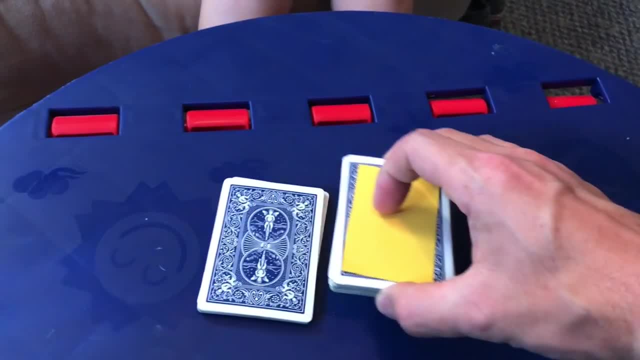 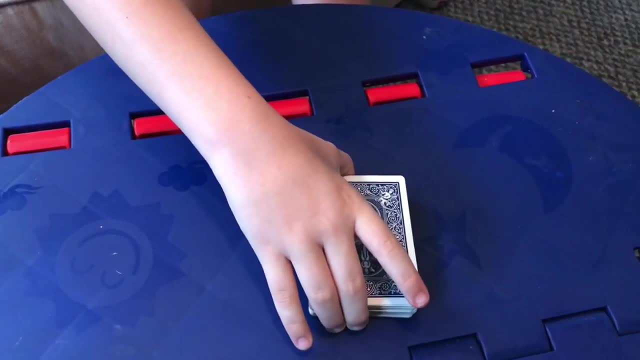 the deck anywhere i want, anywhere you want. it could be anywhere you want, anywhere you want. it could be a little bit, it could be a lot, it could be um, halfway. see, now i'm going to finish the cut. okay, now let's see where you cut to. we're going to flip over. 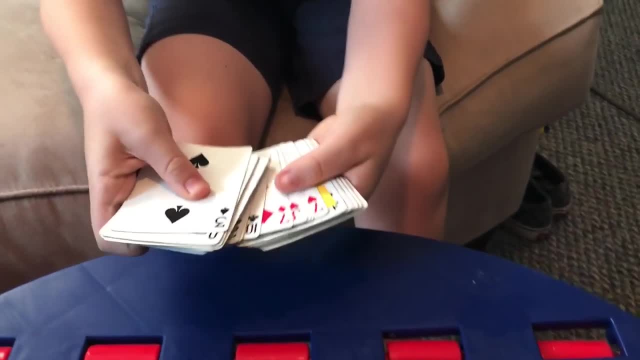 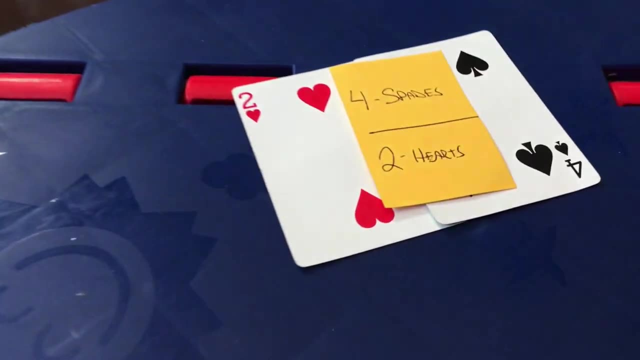 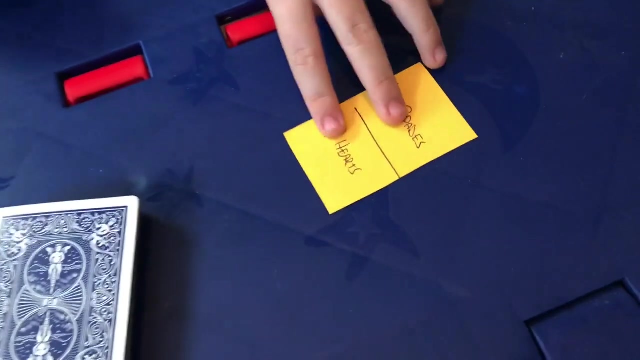 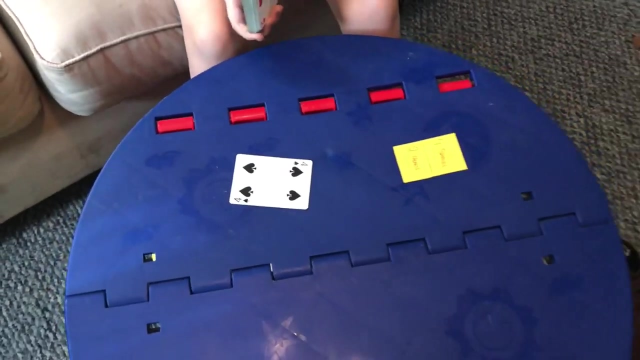 you cut to the two of hearts and the four of spades and that's my prediction. so it requires a little bit of setup. so you want to have your prediction ready before the trick and in your prediction you want to have the two cards that you wrote on your thing on the ends, because it doesn't matter either way. 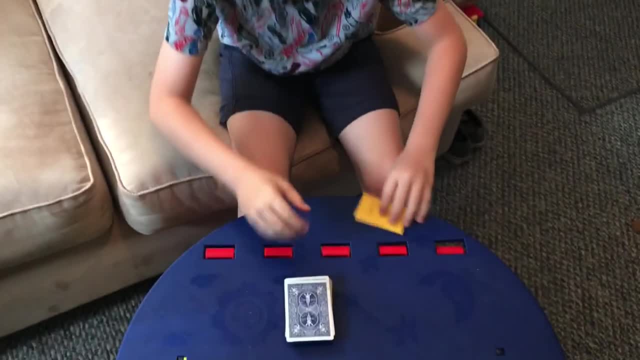 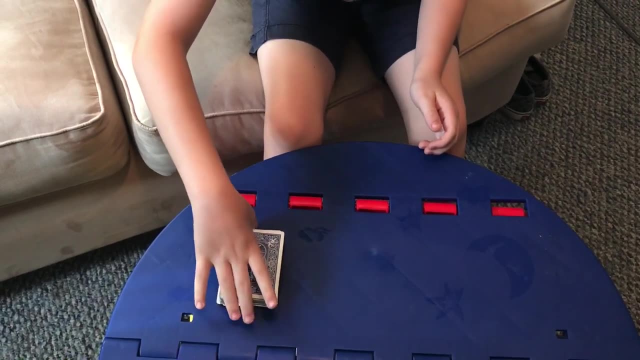 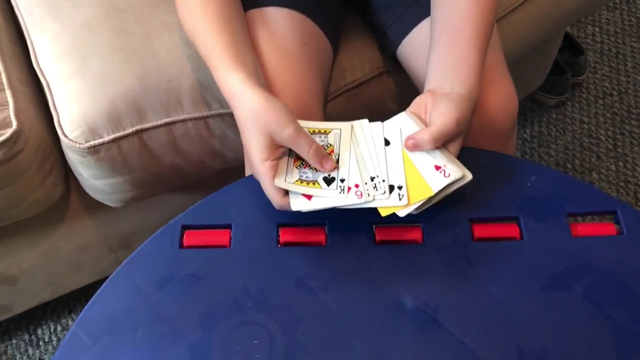 they cut it as long as they're both on opposite ends. you could put this here and i'm just going to leave this up. you, they could cut right here and right here, and every single time. oh, it's always easy to guess the cards, because at the top and the bottom card. 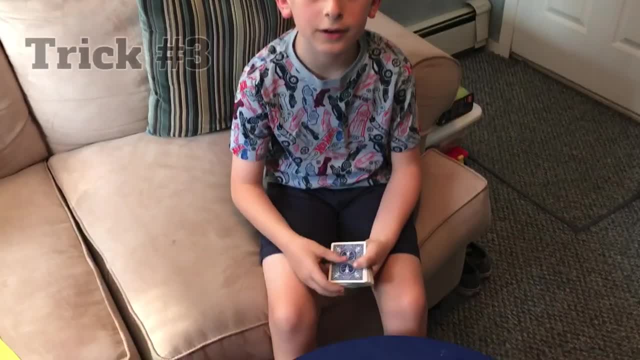 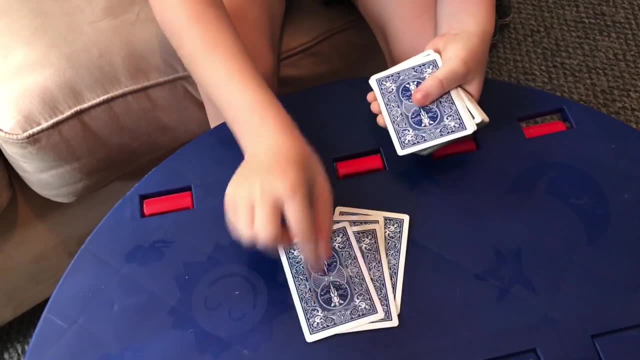 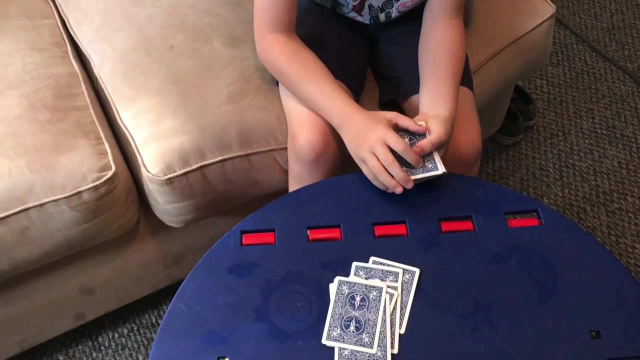 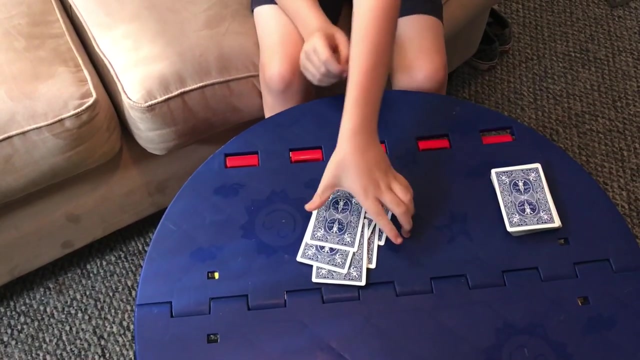 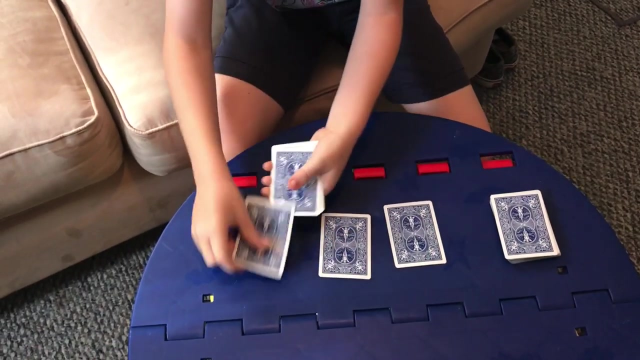 ah, so i'm going to deal the cards and tell me to stop whenever you want. stop, okay. are you sure you want to stop there? uh, no, deal one more, okay, stop okay. okay, take these cards and I'm gonna put them into four piles. What are the odds that?